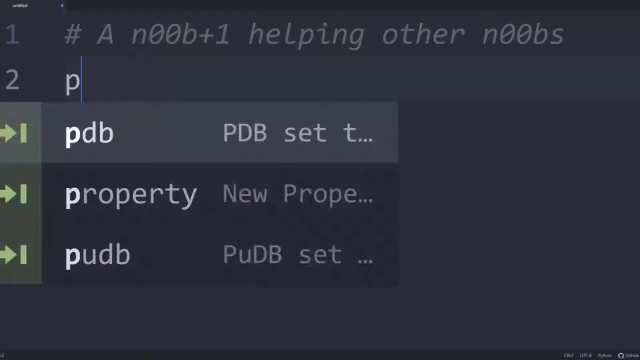 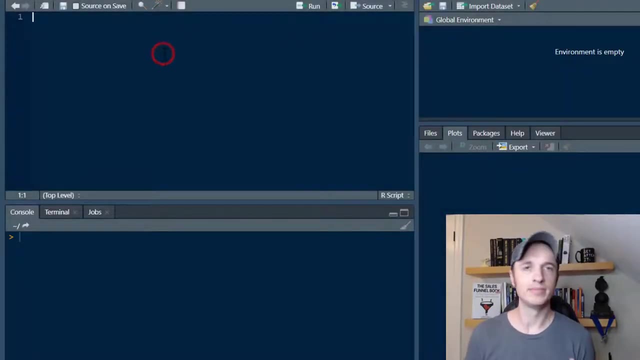 In this video we talk about how to use the aggregate function in R. All right, so let's go ahead and get into it. So, first things first, we need some data so that way we can use the aggregate function with that data. So the data we're going to use for this particular 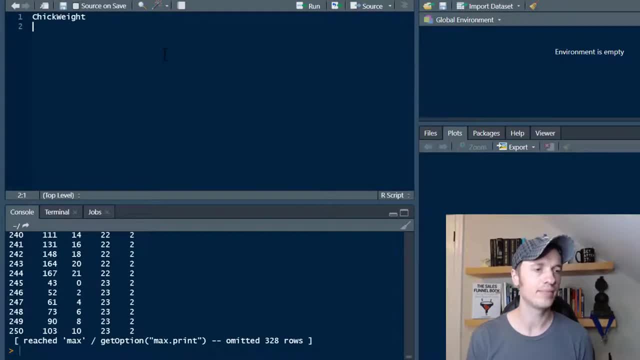 example is the chick weight data, and this data is provided with R studio. So if you have R studio, you probably have the chick weight data automatically loaded into your R studio platform by default and you can load it up by typing in chick weight, just like I did here. 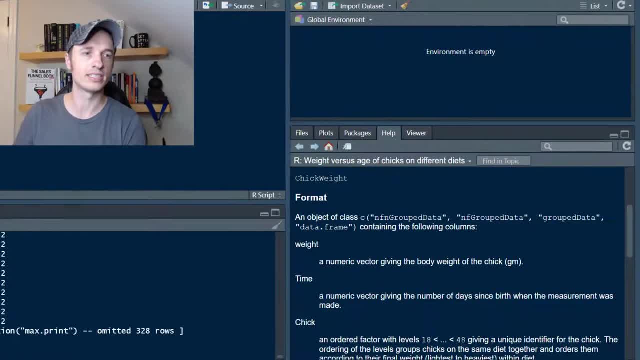 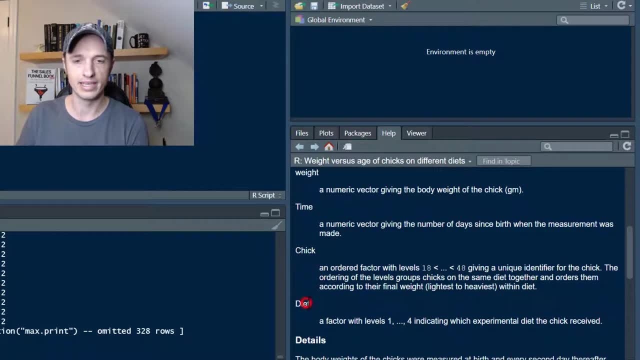 If you want to see what what this data is about, we can go ahead and throw the question mark in there and it gives us a breakdown of the columns. So we got weight, we got time, we got the chick, we got the diet, and then we have some details about the information provided. So, basically, 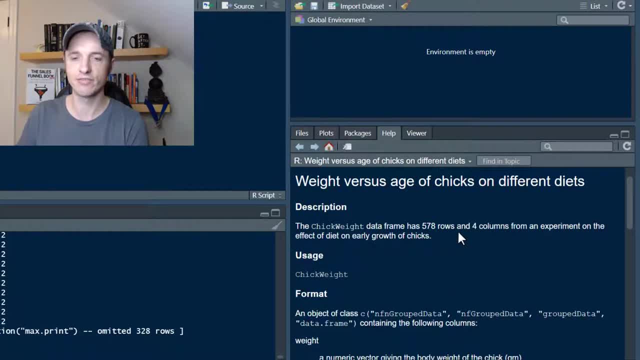 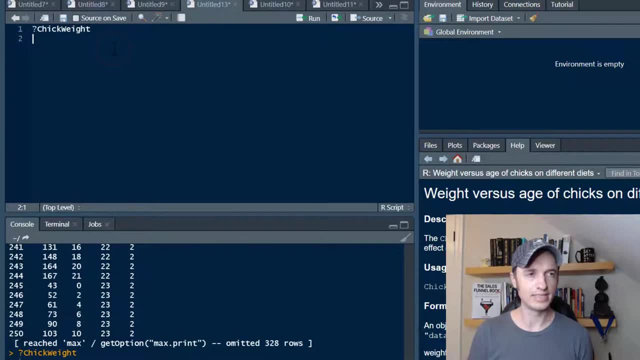 what it's doing is. it's a data frame that has 578 rows and four columns from an experiment on the effect of diet on early growth of chicks. So that's what we're working with right here. Now, just to make things simple, I'm going to go ahead and save this data frame. 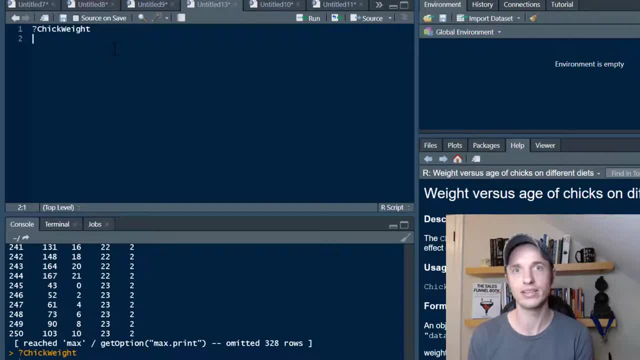 as a two letter variable. so that way I'm not typing in chick weight the whole time. So I'm just going to do cw and then we'll set that as chick weight and we'll store it like that. So now I can call the data frame with just cw. So it saves a little bit of time. So let's go. 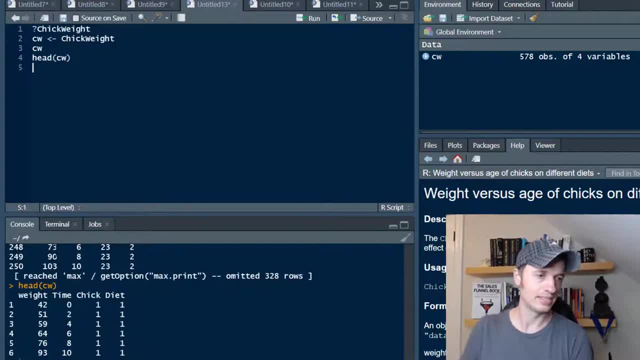 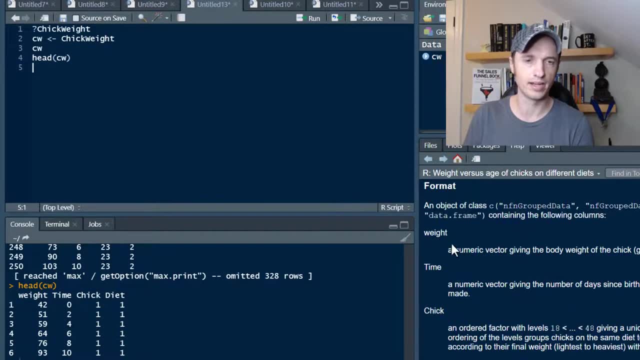 ahead and look at the head. real quick, Head-cw. And so we got the weight, the time, the chick, the diet. So there's what we're looking at here in terms of our columns and everything and what that means, and, for the sake of example, let's go ahead and pull. 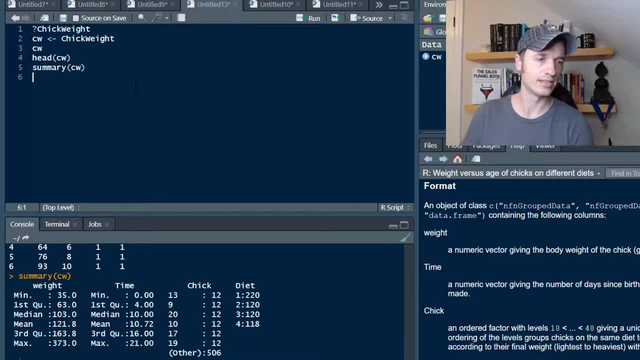 in our summary data. so throw this in real quick. and so now we get our summary statistics for our columns. so here we have it for weight and since it's numeric, we get our minimum, our median, our mean, our max and so on. same concept over here with time chicken diet, our categorical data. so 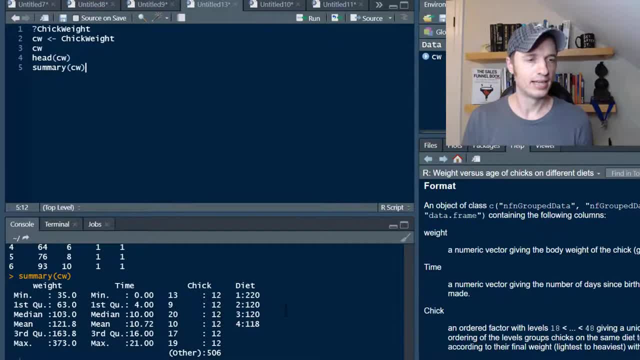 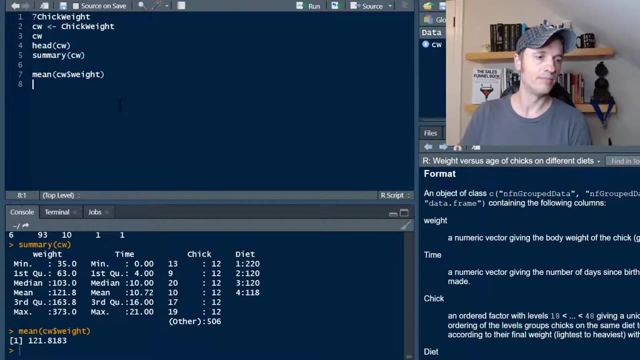 they have it broken down by counts of data that we have, and so now we have a little bit of an idea of the type of data we're working with now. moving on, so you probably know already that we can go ahead and generate the mean of a column if we need to. so, for example, cw and weight will give us the. 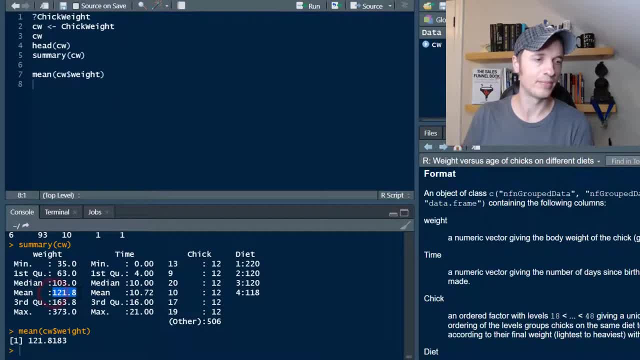 mean for the, the weight column, and we see we get it up here in the summary data, but we also have it broken down by itself down here as well. now where aggregate comes in handy is what if we want to know, like the mean of the weight, based off of which diet they're on. so if they're on diet one, 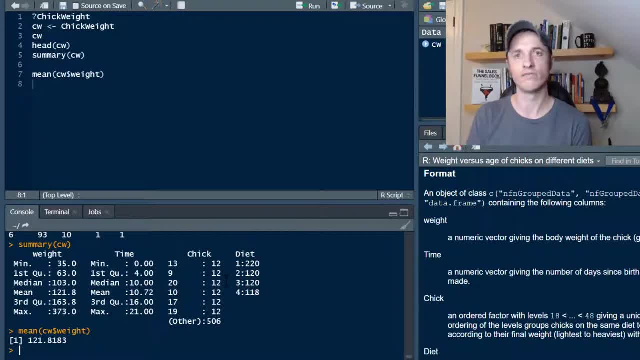 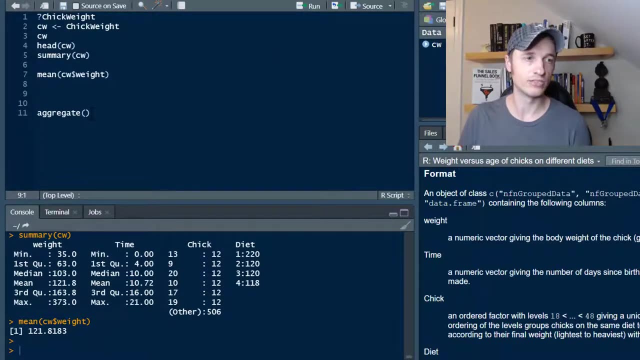 two, three, four, uh, what are the? the average weights for those diets? so we can go ahead and get that with the aggregate function. so, coming on in here, we type in aggregate and then we throw in our continuous variable first, so the one that we're going to get the, the mean of which in our case is weight, right, so let me go. 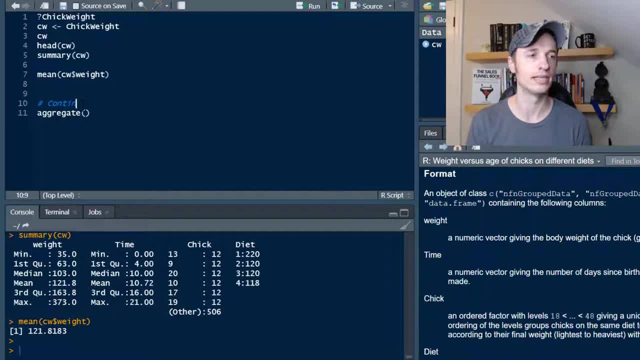 ahead and throw this up here because it's an important concept to remember. so continuous variable first, then categorical variable. so try and remember that with the aggregate function, that's, that's how it works. so continuous variable first. we got weight and we can just type in weight. we don't have to type in the name of our data frame with the dollar sign, we just type in. 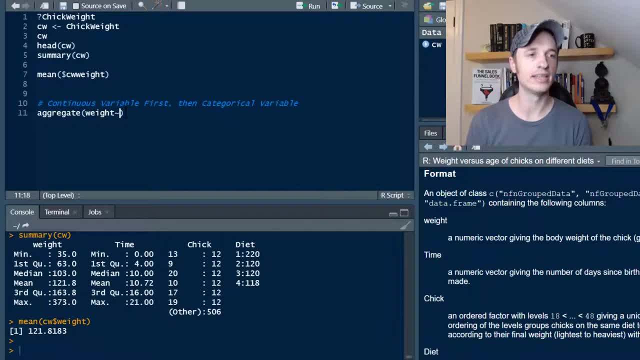 weight, because we'll specify the data next. then we throw in the tilt till day right here. so i throw in the tilde and then we have our categorical variable. in this case it's diet, so type out diet and then the next element or argument we have to add to our function here is our data, in which case 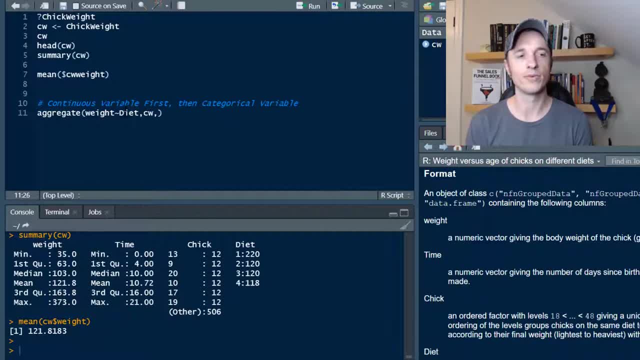 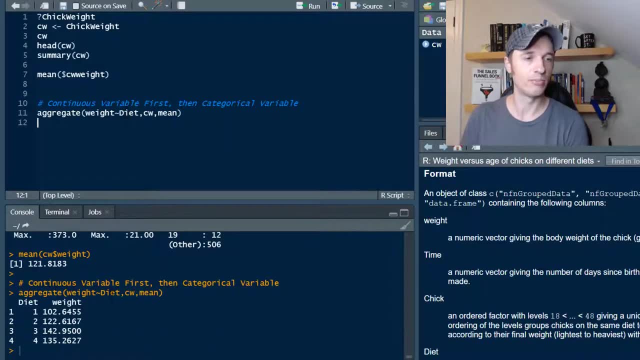 it's cw. and then the next thing, the next, the var previous variable言 we add, is what we wanted to do in our case. we want to go ahead and add them or present the mean. so if we run this real quick, we get a breakdown of the. 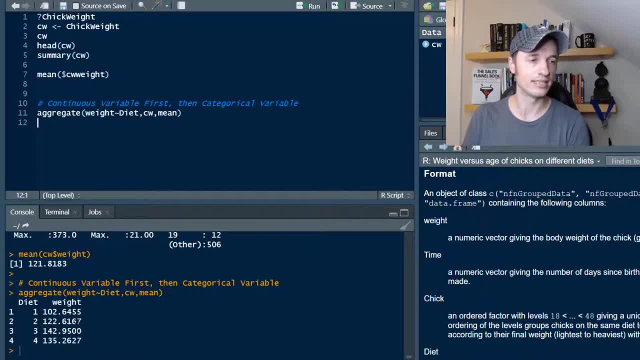 different diets and the average weights for each of those diets. so we can see that it looks like the fattest chickens are on diet number three right, because they have the heaviest weight, and the thinnest chickens are on diet number one because they have the lowest weight on average. so that's pretty cool right now.